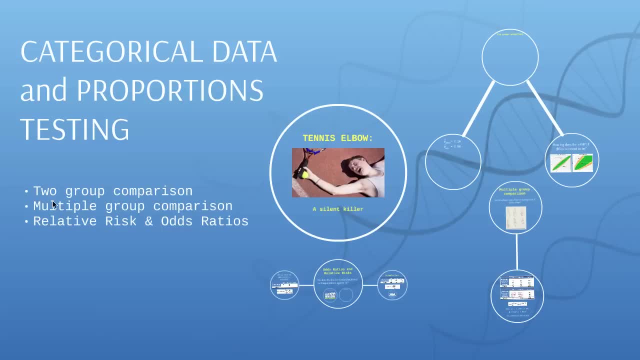 comparing between categorical groups. So a two-group comparison might be to test whether there's a difference between male and female, for example, And then we're going to extend that to a multiple group comparison. so a categorical variable with more than two levels. So that's. 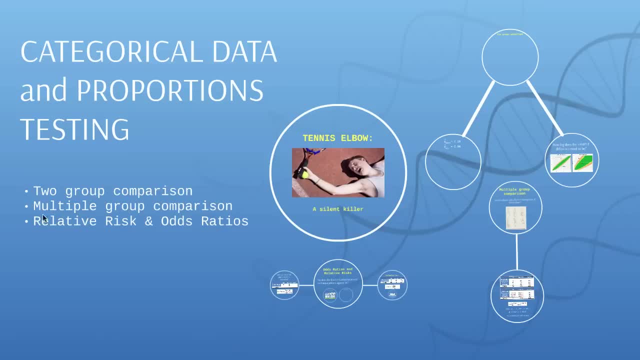 the first half of the presentation. The second half I'm actually going to create its own video, so you might have to skip into the next video to get there, but we're going to deal with relative risk and odds ratios, Which are very familiar terms when you're dealing with health data or, in fact, any data focusing on 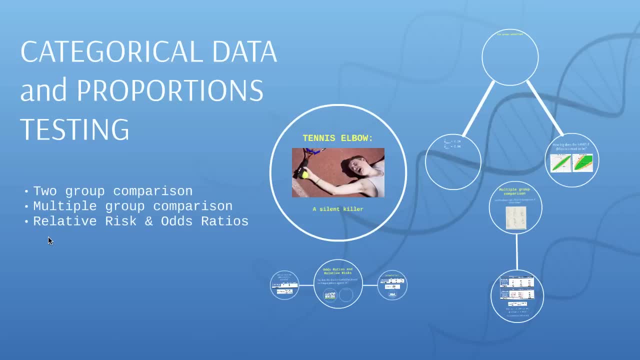 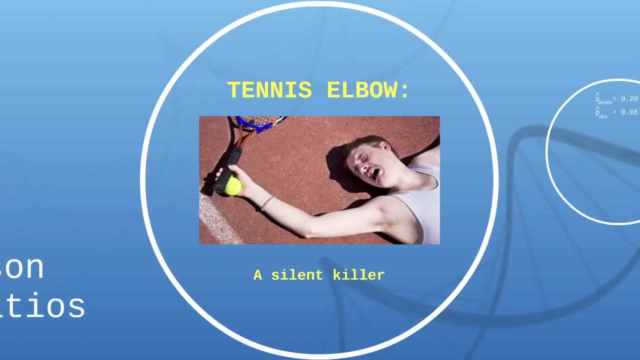 adverse outcomes or adverse events like death or injury. So, without further ado, let's get to my presentation, which is the subject matter of which is to do with tennis elbow. I've called this a silent killer, which it clearly is not, but I thought that photo was hilarious, And so we're. 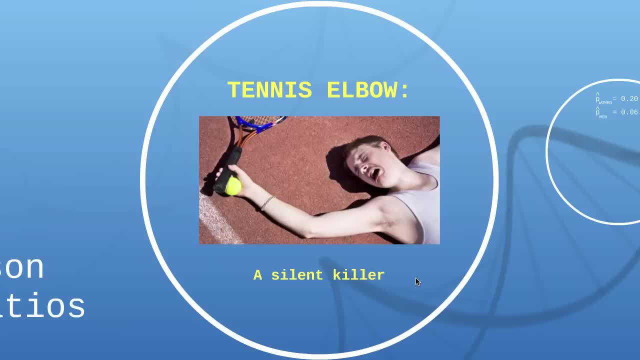 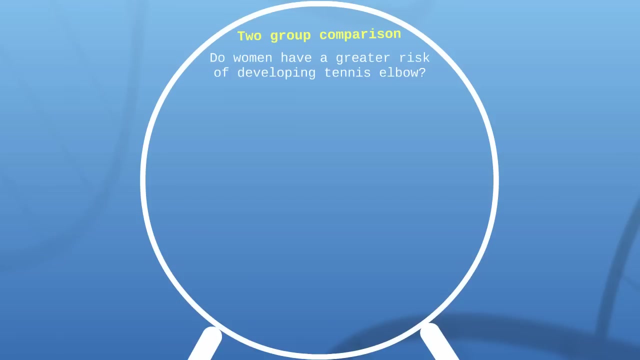 essentially in this presentation, going to be dealing with the risk factors associated with tennis elbow, Which is an actual condition. you can actually look it up. but everything in this presentation is fictionalized- all the data, that is. So, first up, we're going to do a two-group comparison, So we can ask ourselves: here's my 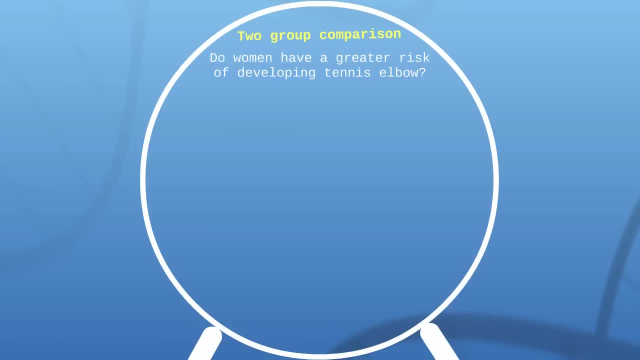 question to you: do women have a greater risk of developing tennis elbow? And so you might think: well, I need some data to assess whether that's the case or not. So we're going to need some kind of sample. Now, before we have a look at the sample, let's just appreciate what we do in statistics In 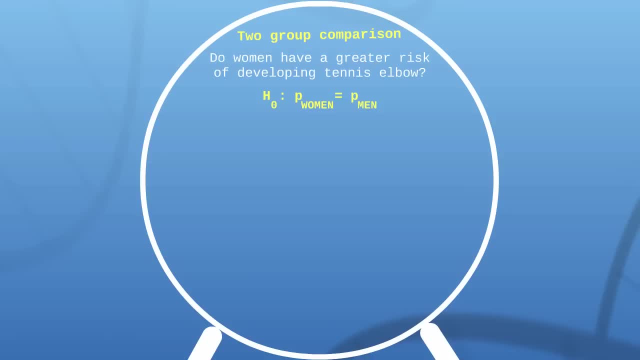 that we always make some kind of conservative hypothesis and put it to the test. So our hypothesis here is that the proportion of women, that's P women, the proportion of women developing tennis elbow, is the same as the proportion of men, And we're going to see whether our sample gives us enough evidence. 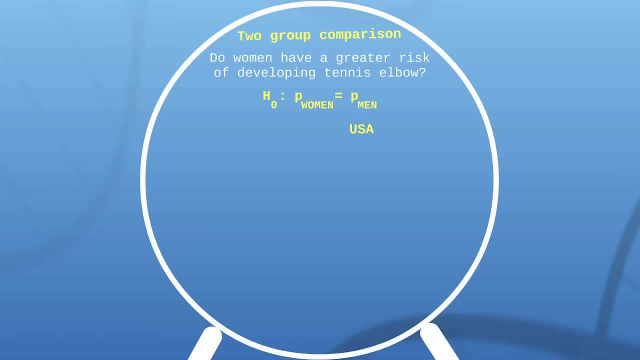 to reject this. Let's presume we have a sample of 200 tennis players from the United States. TE is tennis elbow, So there are a hundred women and a hundred men in our sample And you can see 11 women developed tennis elbow and 10 men developed tennis elbow. 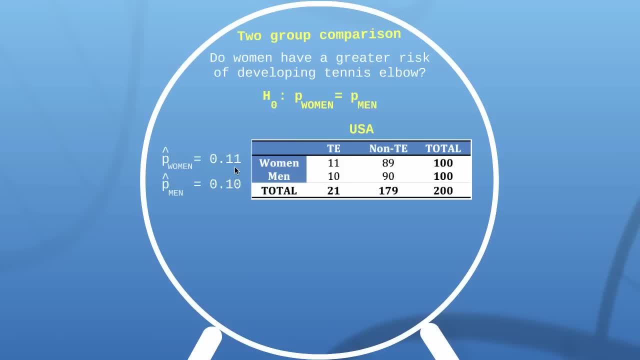 So you can see that from our proportion, we have women at 0.11, a proportion of women it's 0.11 and proportion of men is 0.10.. So, straight away, my question to you is using this sample. 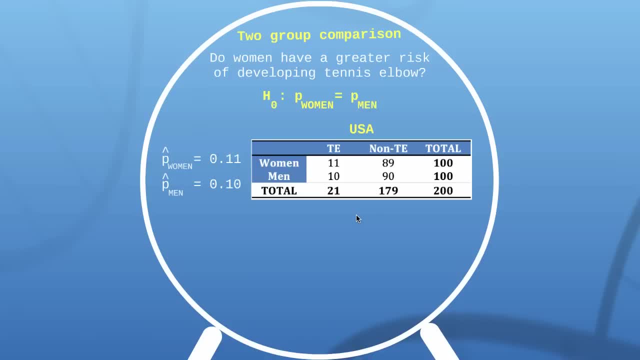 do American women have a greater risk of developing tennis elbow? Your first instinct might be to say yes, they do use. look, it's 11 versus 10.. But appreciate, this is a different study. it's not a appreciate this as a sample, and this difference between women and men could simply boil down to: 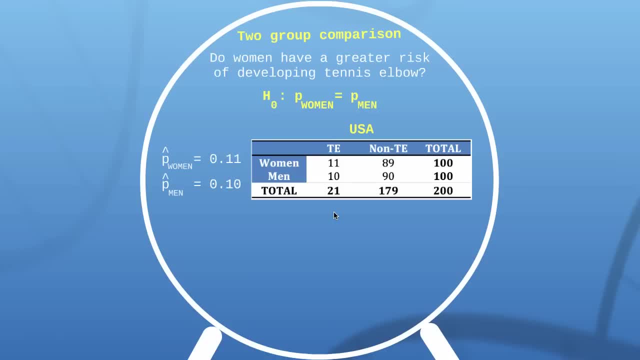 random variation And I'm going to say that those proportions are so close there's no way we're going to have enough evidence here to reject our null hypothesis. We're going to need those proportions to be significantly different for us to even bother with a statistical test. I would say 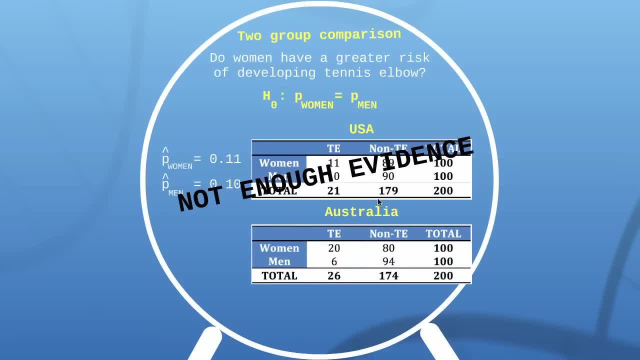 So let's have a look at Australia- Again, completely fictionalized, but you can see that for Australian tennis players the proportion of women gets to 0.2, and the proportion of men is 0.06 who develop tennis elbows. So we've got something to work with here. There seems to be. 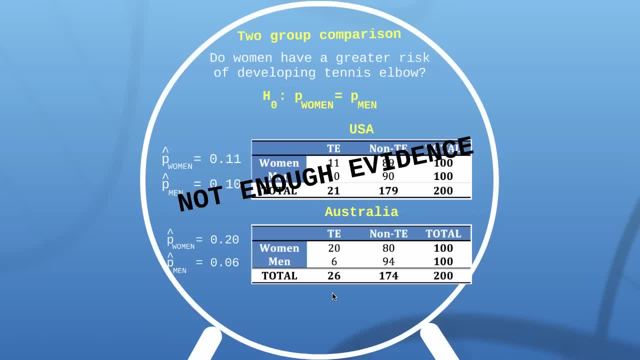 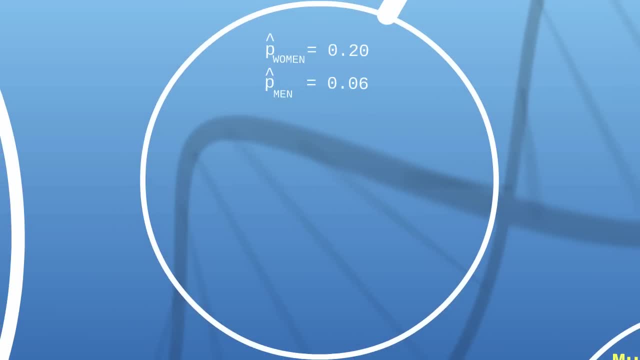 a difference in our sample, and our question is: is that difference large enough for us to infer that there's a difference in the population? So here we go. Here's our Australian sample, and I'm going to repeat that because that's really what I want, drummed home. 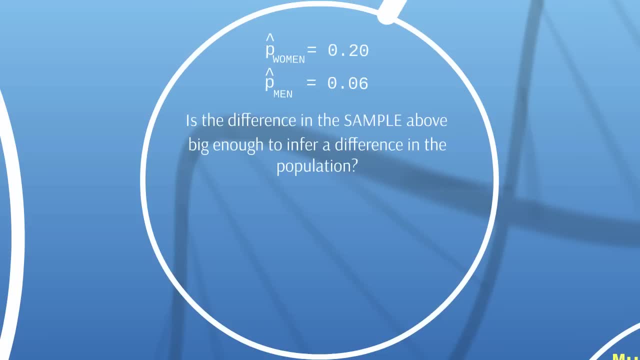 is the difference in our sample big enough to infer a difference between women and tennis players? So let's have a look at Australia In the population. is it so unlikely now that it could be due to random chance that we kind of have to say there's a difference at the population level? Now I don't know how to answer that. 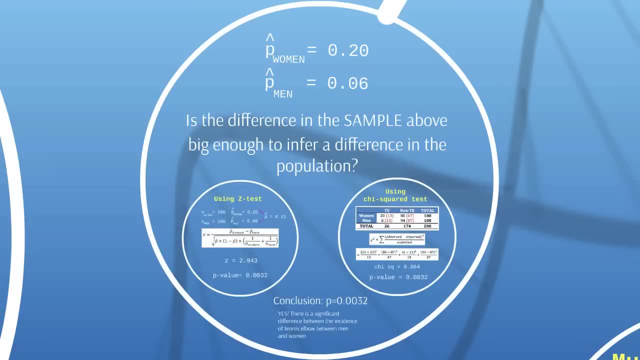 question just by looking at it. so we're going to have to use some kind of test to see whether that difference is large enough, And there's actually two different tests we can use, The first of which is a Z test. What we need to start is just the number of women in the sample. 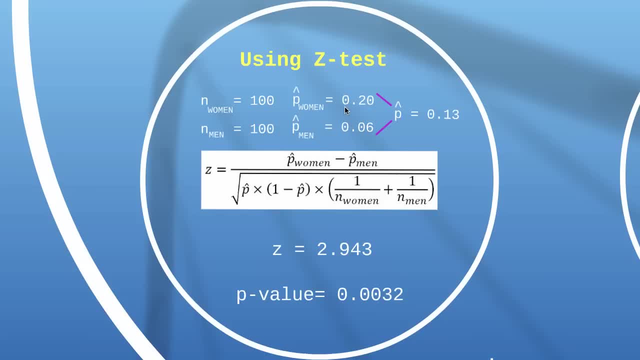 the number of men. and we have that, The proportion of women developing tennis elbow and the proportion of men. And we also need this sample-wide proportion. So, conveniently enough, the number in both of these categories is equal, So we can just. 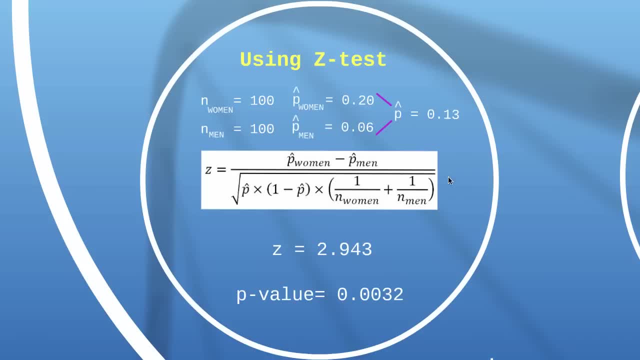 take the average of 0.2 and 0.06, and we can plug all this information into this formula, which essentially just assesses how big the difference is between women and men developing tennis elbow, And we get this Z score of 2.943.. Now, that's essentially a measure of how extreme 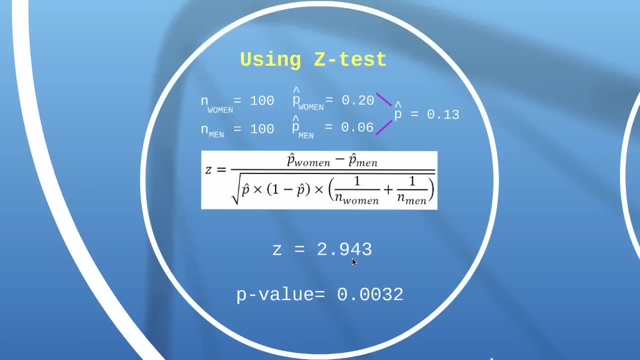 our sample is under the null hypothesis. I really want you to think about what I just said there: how extreme our sample is, given the null hypothesis. Now, that null hypothesis is that there's no difference between women and men, and we had a sample that had quite a big variation. Now how? 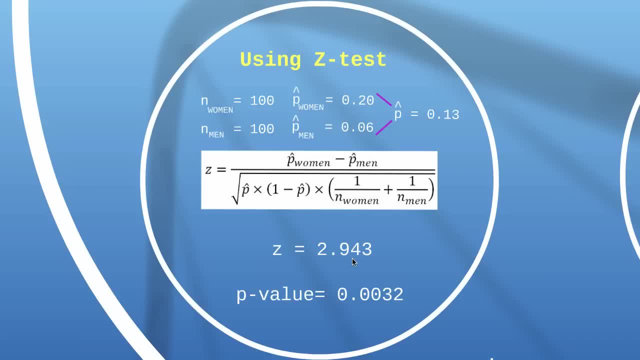 extreme was our sample, if we presume it came from a population of equal proportions. Well, the actual magnitude of this value is not so helpful. so we developed this thing called a p-value, Which you can calculate straight from this Z score. You can do it with Excel or any kind of. 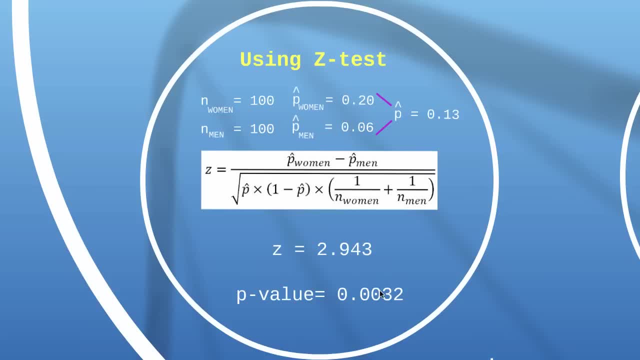 statistical software. Usually they just give it to you if you run any kind of software with a Z test in it. And what this 0.0032 says is that the chance of getting a sample as extreme as the one we actually got is 0.0032, if we assume the null hypothesis is true. So that does budge our 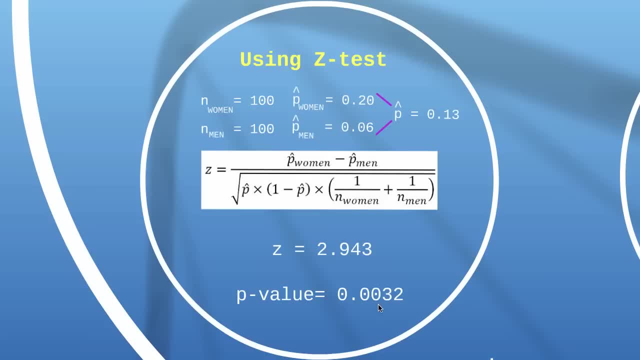 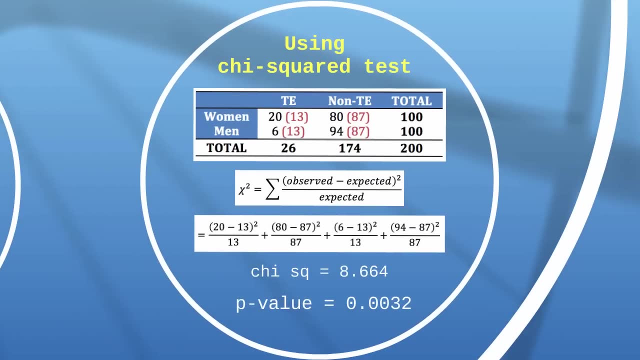 confidence in that null hypothesis, And that's what we're going to do. So we're going to do a null hypothesis. We can infer that there's a difference between men and women. Now let's have a look at the chi-squared test, using the exact same information, but just coming at it. 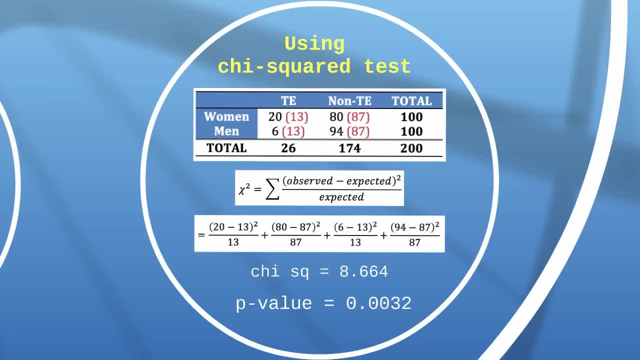 a different way And, as we'll find out later, this is actually very useful when you have more than two categories. So, very briefly, the way you'd conduct a chi-squared test is to generate these expected frequencies within each of these cells. So the black text is what we initially saw, That's. 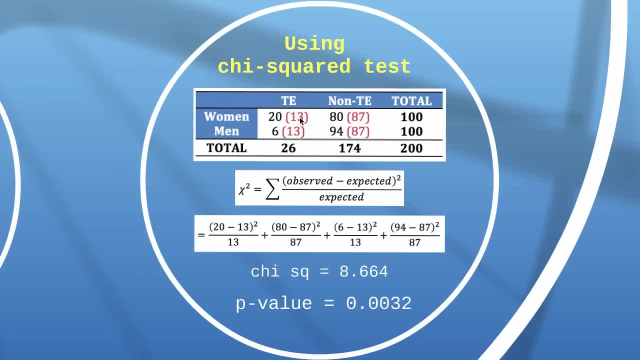 what I've calculated as what would be expected under the null hypothesis, under the hypothesis that there would be no difference between men and women. And it's relatively simple to get these values: You essentially just multiply the two marginal values together and then divide by the. 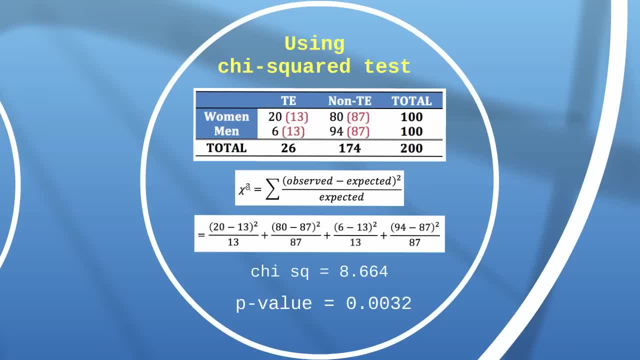 total. Anyway, now the chi-squared test essentially compares the observed values to the expected values under the null hypothesis. So again, it's kind of seeing how extreme our sample is if we assume the null hypothesis is true. So we're going to go 20 minus 13 squared divided by 13.. And 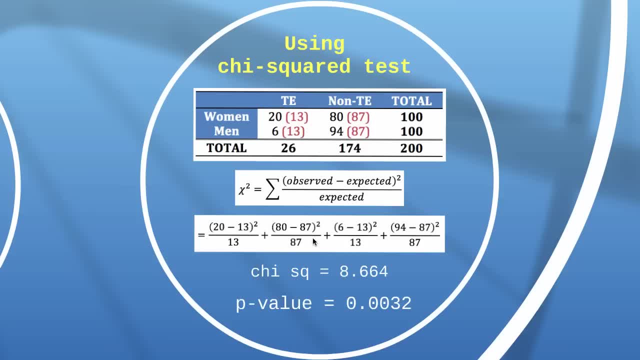 we're going to do that for each cell of this table. Now, I tend not to put too many formula into my videos, but I think this is really important, because you use the chi-squared calculation everywhere in statistics, And this is. if you've not seen it before, this won't be the last time. 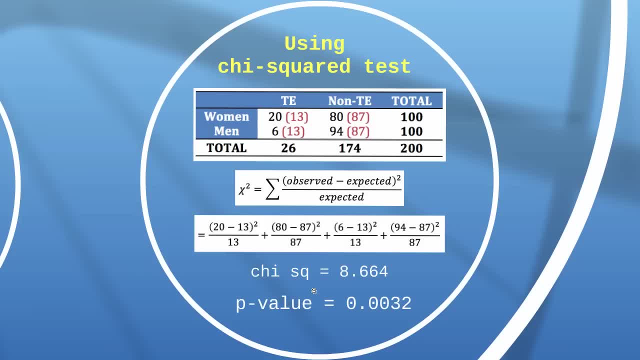 you'll see a chi-squared stat, I promise you. So here we have a chi-squared statistic of 8.664.. And again we can try to find the p-value derived from that chi-squared statistic. And there's just. 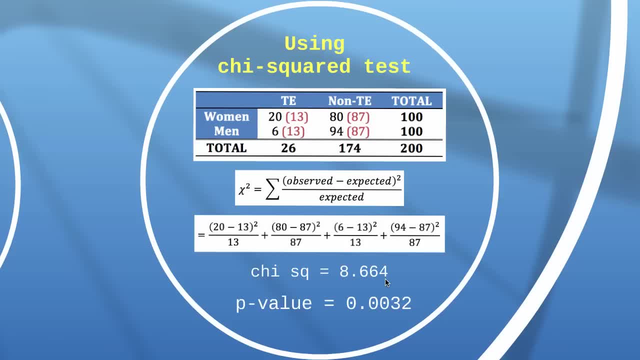 a little side note. Unlike the z-statistic, the chi-squared statistic also has this extra feature called the number of degrees of freedom that we need to take account of. I won't go into degrees of freedom too much, but in a 2x2 table there's going to be one degree of freedom, And in any kind. 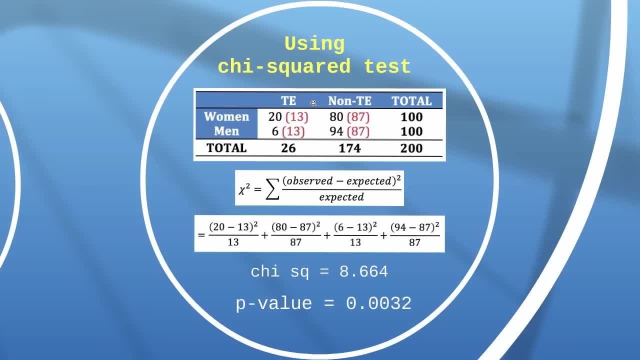 of contingency table as we have here. the way you calculate the number of degrees of freedom is just the number of columns minus one. So here's the columns minus one. So there's two columns. Columns minus one is one. You multiply that by the number of rows minus one. So again by one, So one by one. 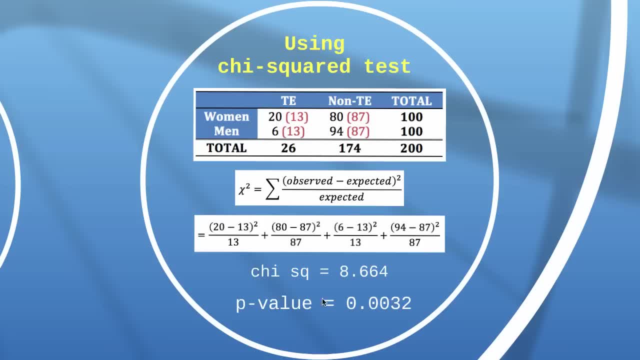 is going to be one. So the p-value for a chi-squared statistic of 8.664 is 0.0032.. No surprise, It's exactly the same as for the z-test we just saw. So our conclusion is that there is a 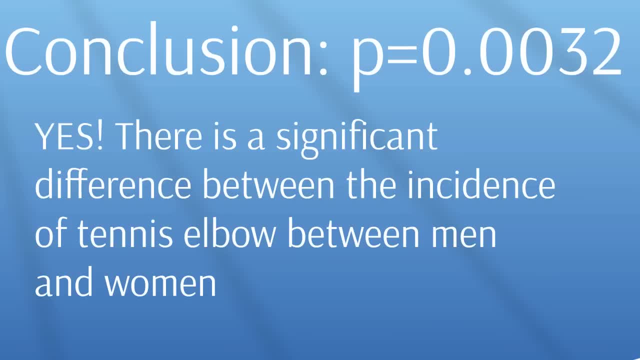 significant difference between the incidence of tennis elbow in men and women, And that's why we don't use the p-value for men. Why? Because our p-value is extremely small At any level of significance- 99%, 95%- we would be rejecting the null hypothesis, So our sample was just too. 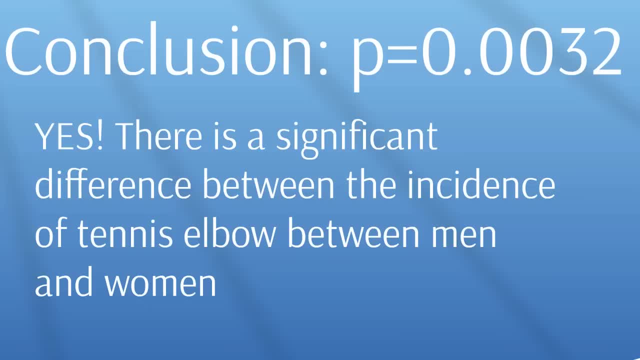 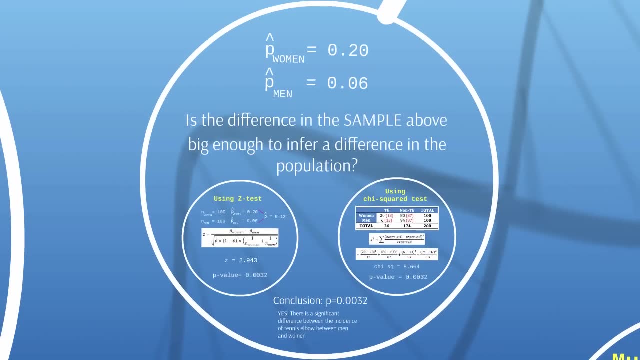 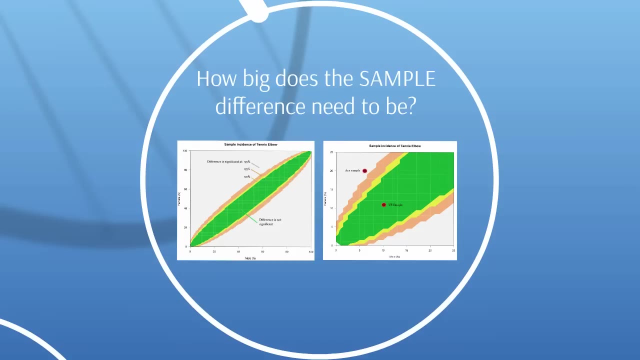 extreme to realistically hold on to that hypothesis that there was no difference in the population. Now this is a little bonus section for the two-group comparison. We're kind of interested to see how big that sample difference needed to be for us to reject the null hypothesis, Because remember, with that United States example it was so close we were. 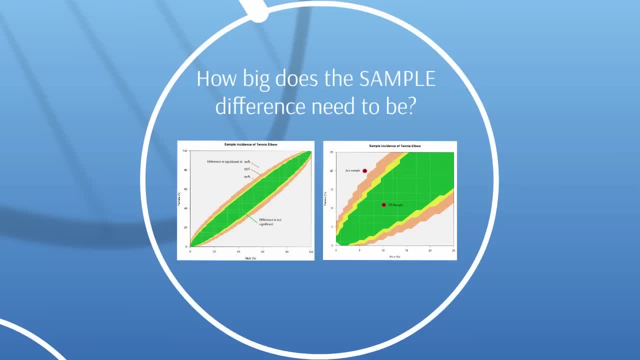 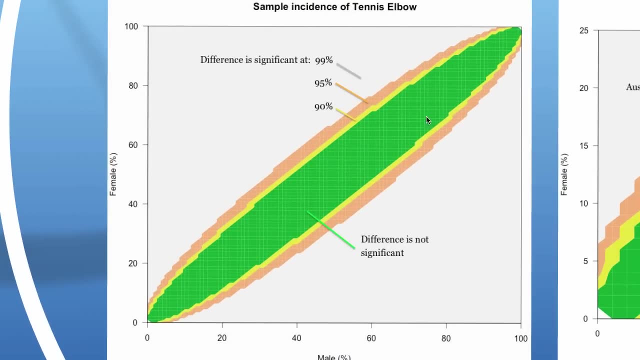 like. there's no way that we could possibly reject the null hypothesis And for our Australian example, we did reject it. So if we look at these plots that I've put together, you can see the green area in here is where we are not rejecting that null hypothesis. And have a look at the axes here: The 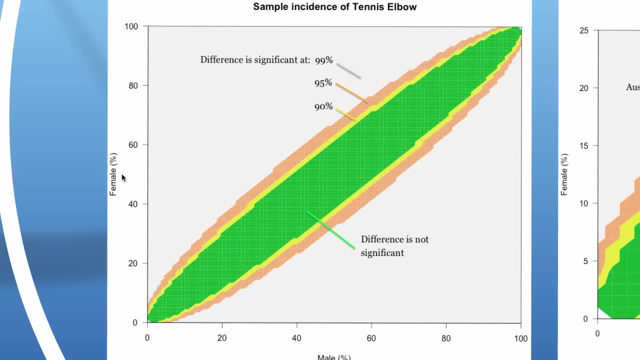 bottom is male. Sorry, it might be cut off slightly. The vertical axis is female. So if 20% of your female sample and 20% of your male sample you have tennis elbow, then you're going to be well within this green region. 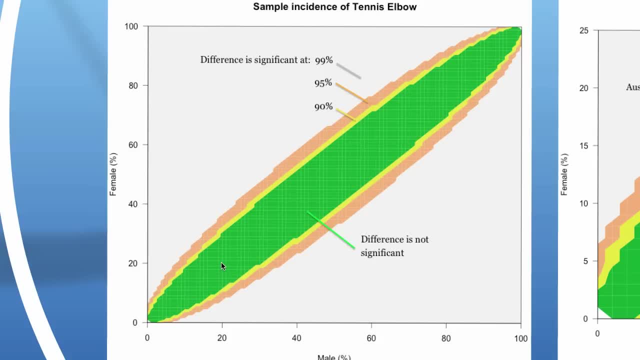 and you're not going to be able to reject that null hypothesis. So essentially that difference is not significant. But as there becomes a difference between the male and female proportions or percentages, you're moving into this yellow and then peach and then gray territories here, each of which represents a rejection of that null hypothesis. 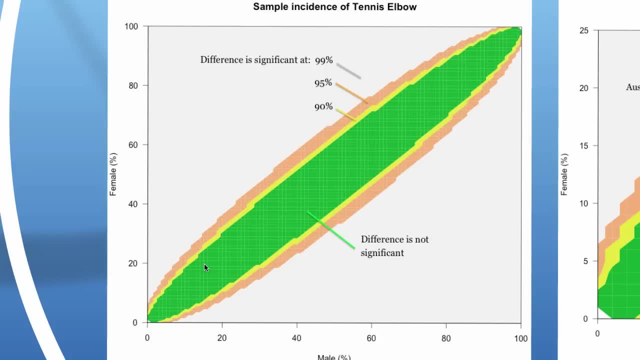 different levels of significance. So why I put this plot together was that I was keen to see what the effect was when the proportions are low versus when the proportions are close to 50%. And in our case we're just sort of looking at this bottom section here, this bottom fifth of 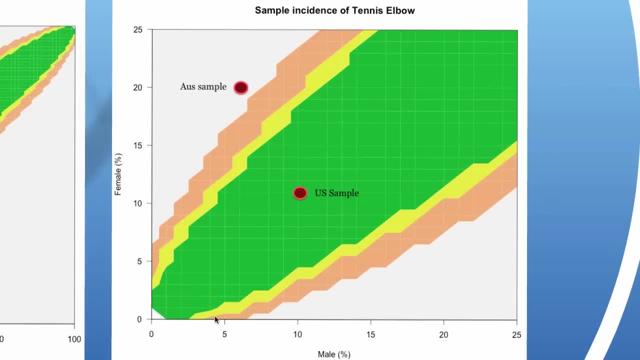 this plot. So if we blow that up, we can see that where we have our two samples, there's our Australian sample with, I think what, 6% for male and 20% for female, And here's our US sample with 10% and 11%. So clearly we knew this before we even tested it, but there's no way we're going to. 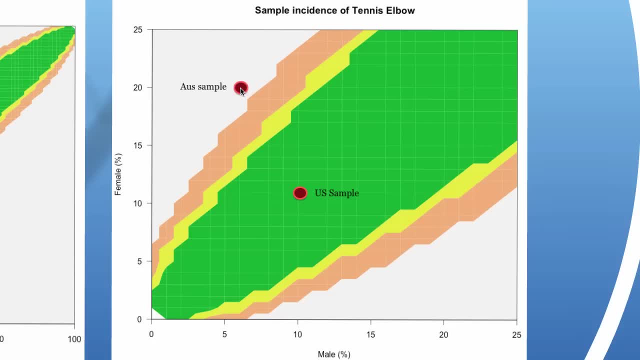 be able to reject from that US sample, whereas for Australian sample it was in that rejection region. So what's interesting about this is that when your proportion is quite small, for both male and female respectively, the difference doesn't need to be as large as when the proportion is sort of closer. 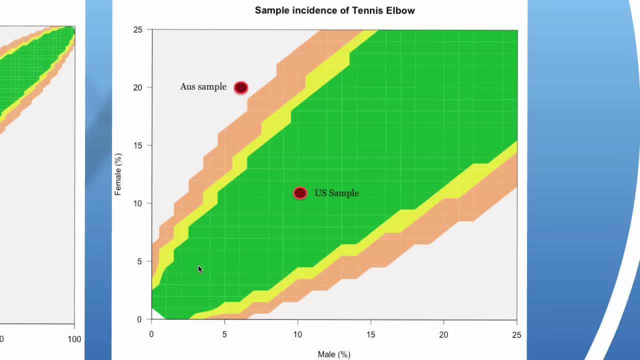 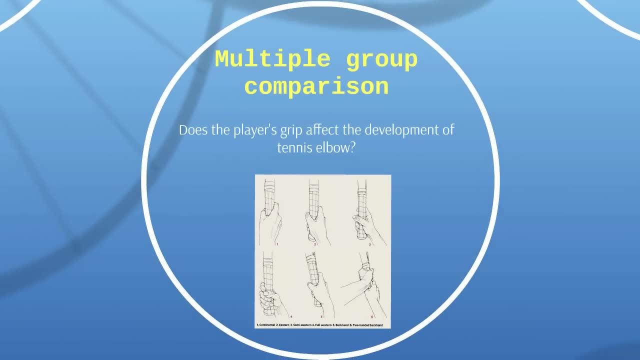 towards 50%. Maybe that's mildly interesting, but I thought I was keen enough to see how that played out. All right, so let's see now how we would make a comparison across a group that has multiple levels. So in this instance I'm asking: does the player's grip affect the development of tennis elbow And 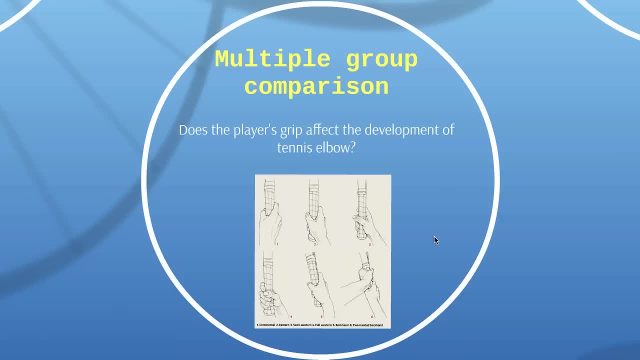 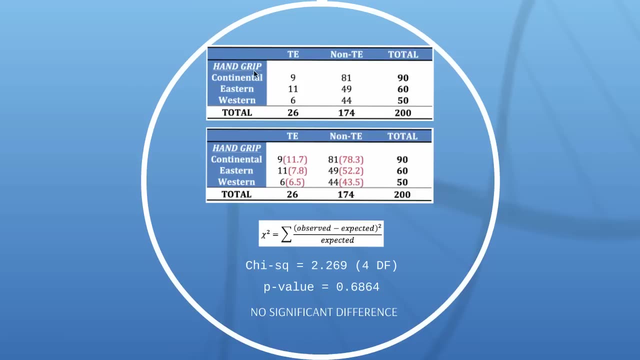 here's a little plot of the various grips you can have on the racket. So again, let's take a look at this particular sample. This is the Australian sample again, but instead of looking at males and females, we're ignoring gender for the moment- and just looking at what hand grip they use to hold. 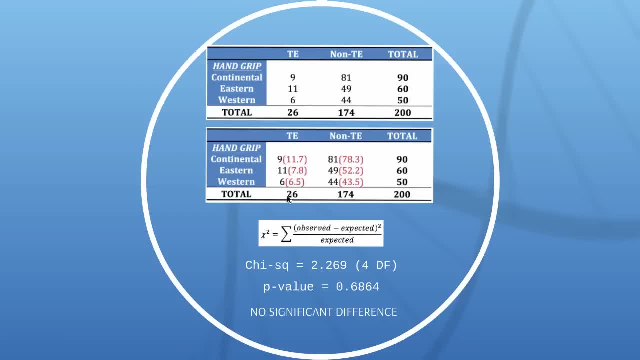 the racket And much like the method we used for the chi-squared test in the comparison between two groups. we're going to use the exact same method, but it's between three groups, So we've got to try to find these expected values for each cell, given complete independence between the hand grip and